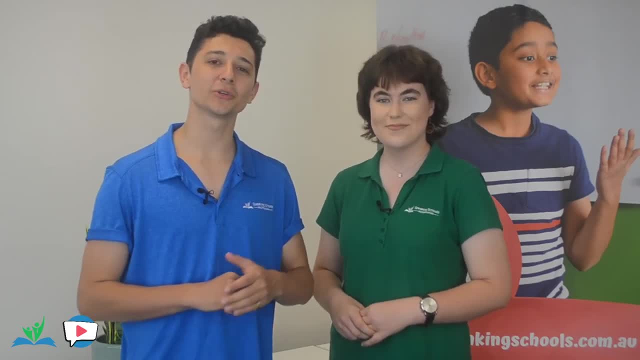 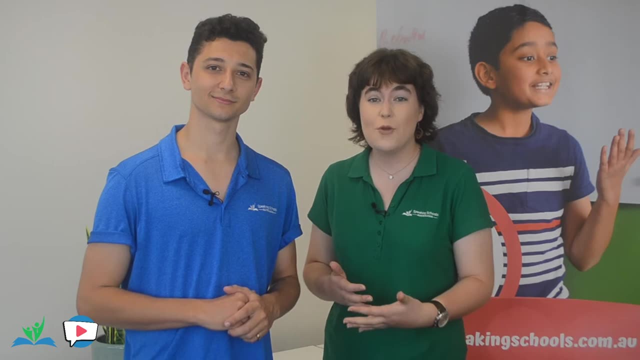 Hi parents, With the school year just starting up again, we know that you and your child must be excited for the upcoming public speaking opportunities. We also know that it can be a bit hard at times to know the best ways to help your child practice their speeches. 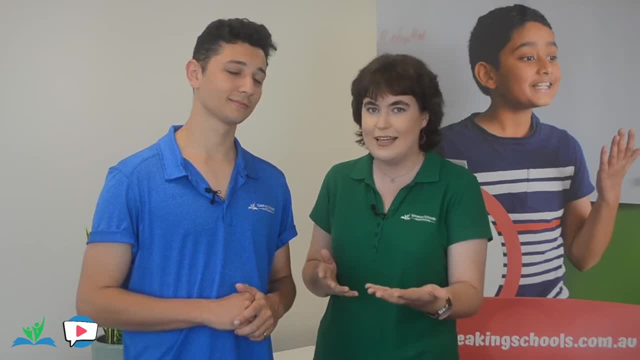 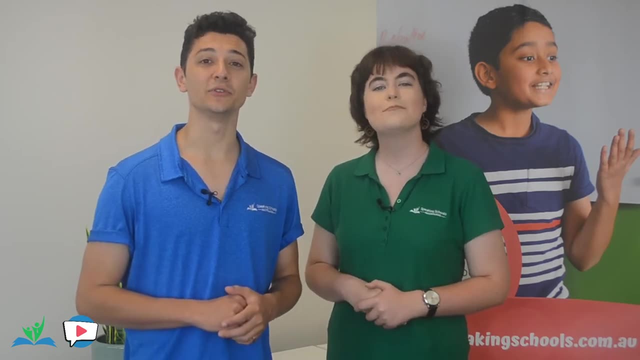 and prepare for competitions, Because, let's face it, if we don't know what we're doing, public speaking can be a bit nerve-wracking, even from the sidelines. So in today's video, we're going to give you some tips on how to help your child. 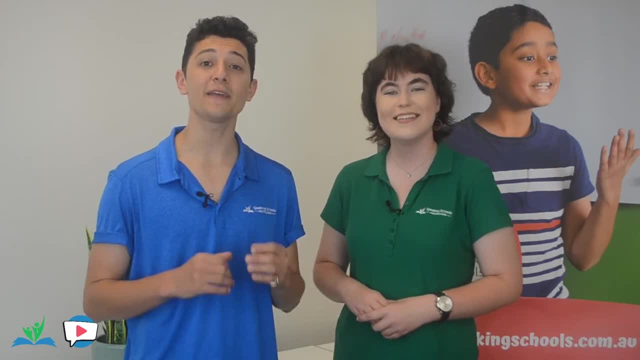 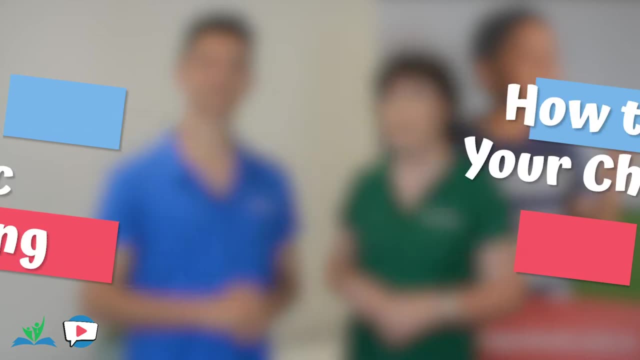 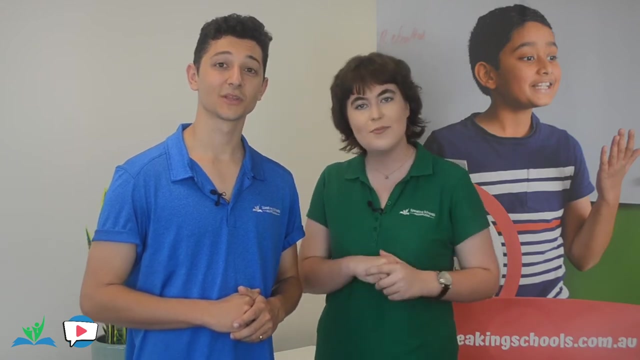 based on the real-world experience of the coaches at speaking schools on what they've found to be most useful for them. Now there are a lot of different ways that you can help. You've just got to work out what works best for you and your child. 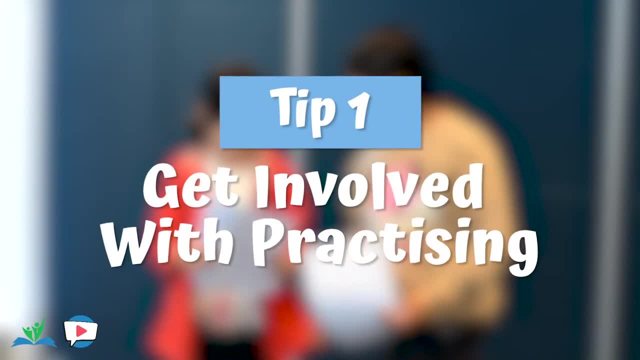 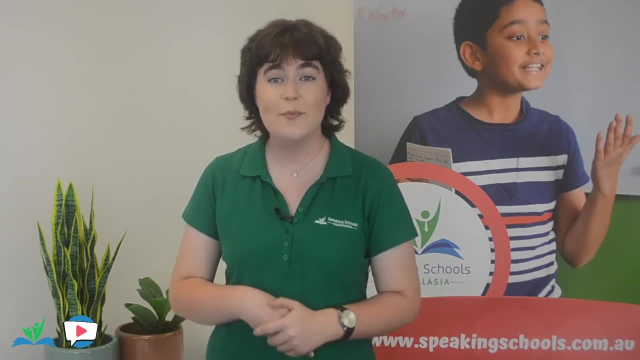 So let's get into it. Here are our top three tips. One of the best ways to build confidence with public speaking is to get your child practicing out loud. Plan a time in the week where you'll sit down and listen to your child practice. 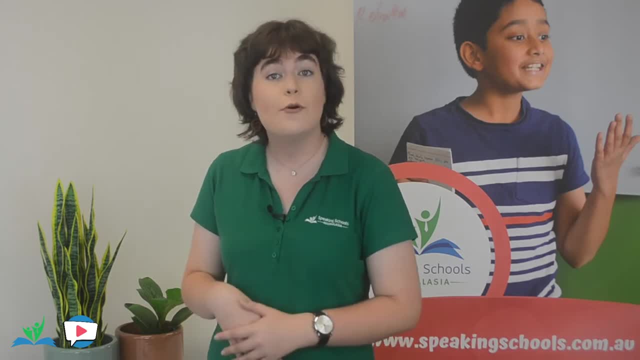 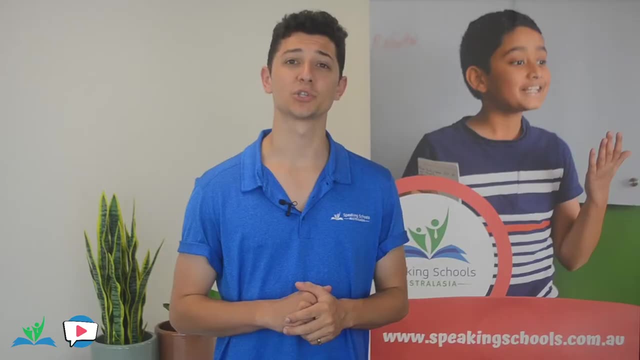 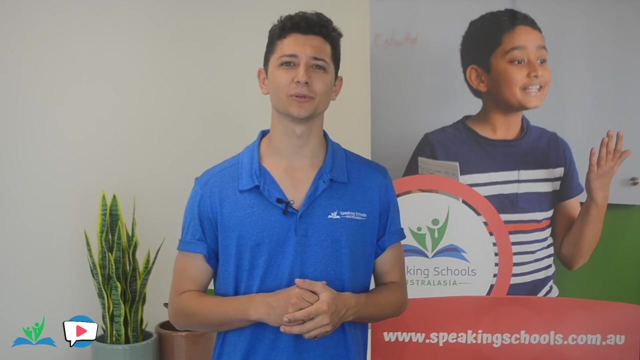 It's a good opportunity at these practice sessions to work on small things too. Is there enough eye contact? Are they speaking at the right pace or the right volume? Even checking something as simple as does this speech make sense can help iron out the speech before they're actually presented to an audience. 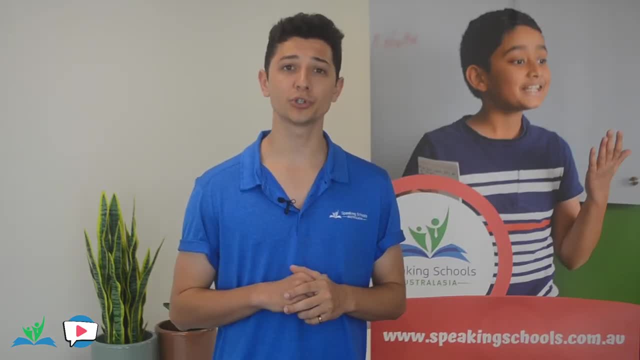 A lot of public speaking competitions have an impromptu speech section where students will get a very generic topic prompt and have to come up with a speech to present in only a couple of minutes. That's why it's great practice, while on the drive to school or to sport, to choose a topic. 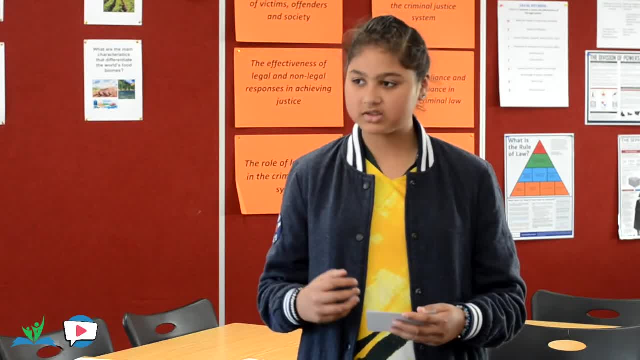 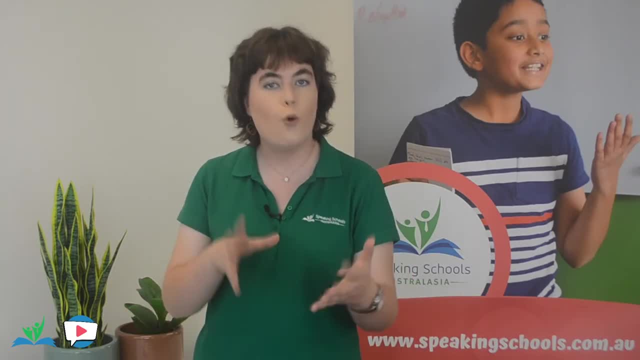 and get your child to say as many good things and bad things as possible about it. This will help generate ideas and arguments they could use in a speech. This can also be really useful when listening to or watching the news. Current affairs can make great prompts in speech and get children thinking about the world around. 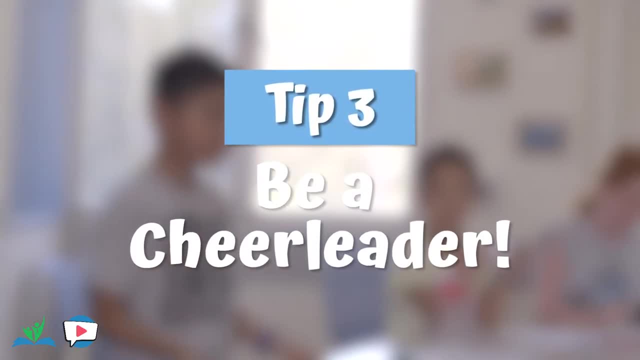 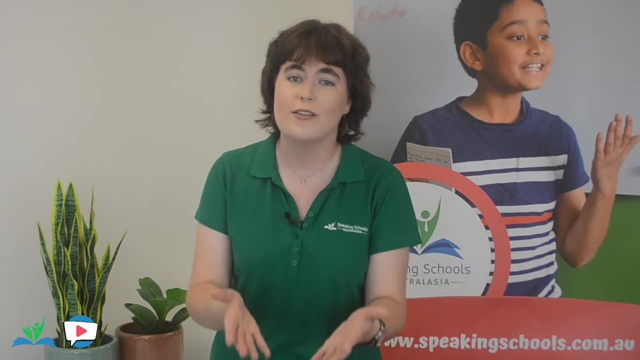 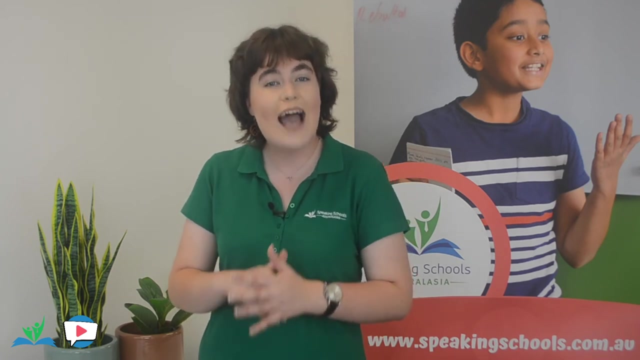 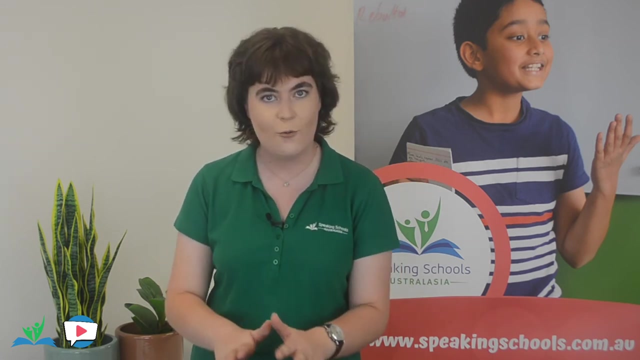 them. No matter whether someone is doing their first speech or their 40th speech, everyone still gets nervous, So positive affirmation and encouragement can go a long way to boosting their confidence and getting them in the right headspace. My parents would always remind me that it was just a competition and not the end of the world.